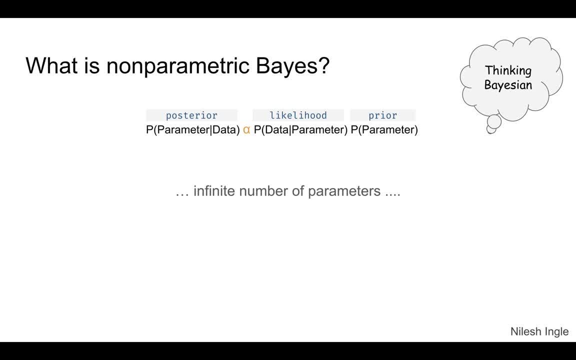 what we are trying to find are the parameters that best represent the data in a cluster, the cluster data points. So to find those parameters, we start out with a prior, which is a prior belief of what the values of those parameters could be. This could be the mean and standard deviation. 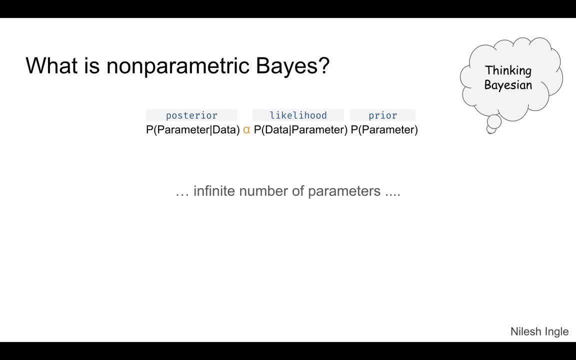 Now, to get that prior, we can sample it from another device distribution and then in presence of the data. so after we see the data, which is going to be the likelihood, how does that update our belief in the prior? that is to say, we find the posterior with the information that we get after looking at. 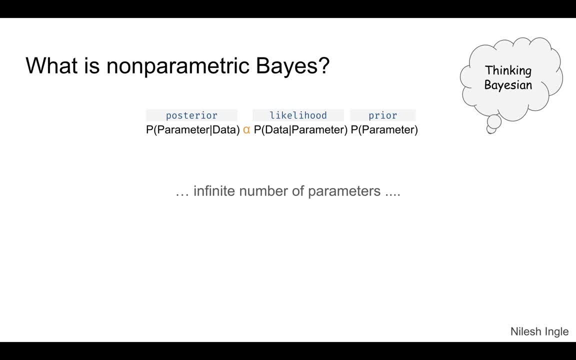 the data. so that's the whole thinking behind what we are going to discuss now. it's based on this particular part right here, so the posterior is proportional to likelihood into prior. so we have some idea about what the data should, what the parameters should be to represent the data that we have here, and that's. 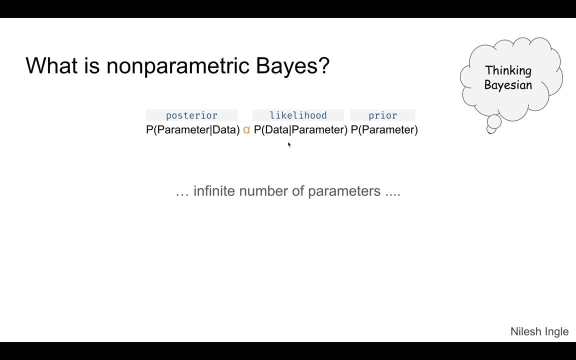 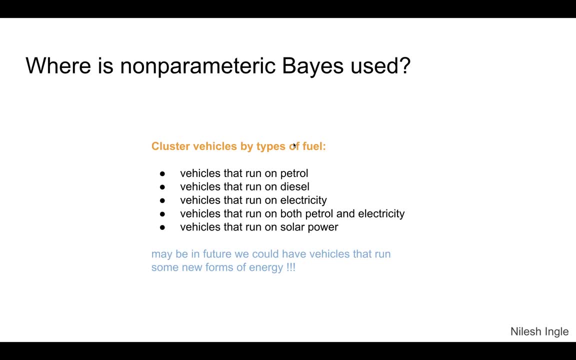 what we are trying to maximize is this particular part, likelihood- and where then this non parametric Bayesian methods are useful. so here is a very crude example. let's say we have a cluster, we have data and we are trying to cluster vehicles by their fuel type, so the vehicles could. 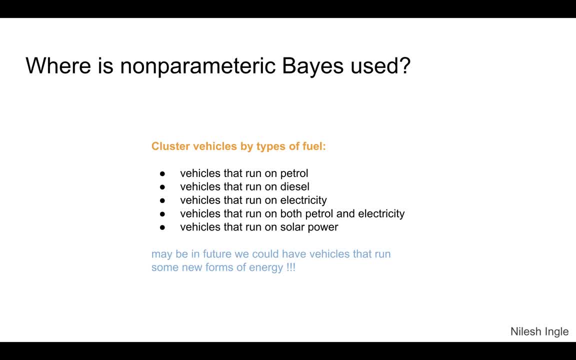 be running on petrol, gas, or they could be running on diesel, electricity, or they could be hybrid vehicles running on petrol and electricity, or they could be running on solar power. and let's imagine a hypothetical situation where every month, there is a new technology that is being developed that adds a new type of fuel source to run a particular vehicle, and so each month we are 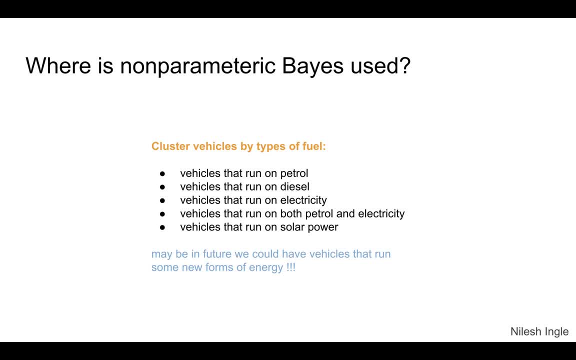 getting a new fuel type that can be used. so, as the data comes in as the year progresses, we'll have a new fuel type that can be used. so, as the data comes in as the year progresses, we'll have a new fuel type that can be used. so, as the data comes in as the year progresses, we'll have 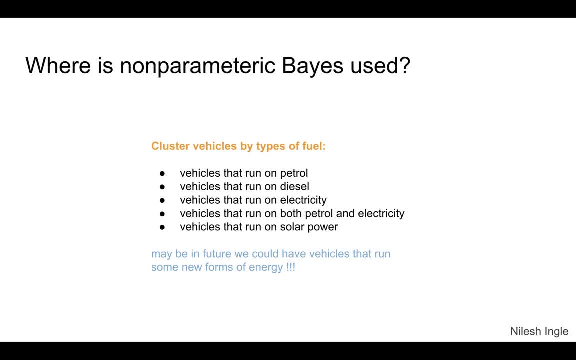 new clusters to be found that are not yet known on the present day. see what i'm saying. so what we are trying to find is if there are unknown clusters that may come up in the future, but we can prepare a model that takes into account what those takes into account or creates room for. 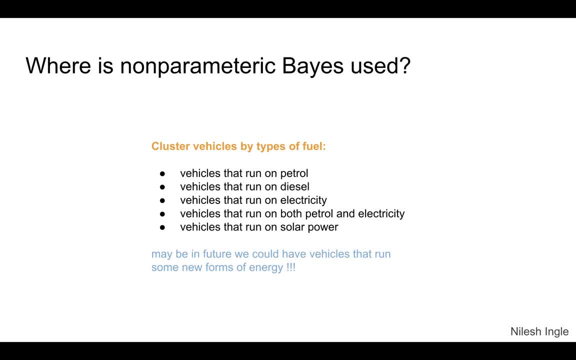 those unknown clusters ahead of time. so when they are do appear, the model is able to work with those new, newly added cluster data as well. another example is, let's say we are trying to segment people based on their interests. so let's say, in the month of january, the interests. 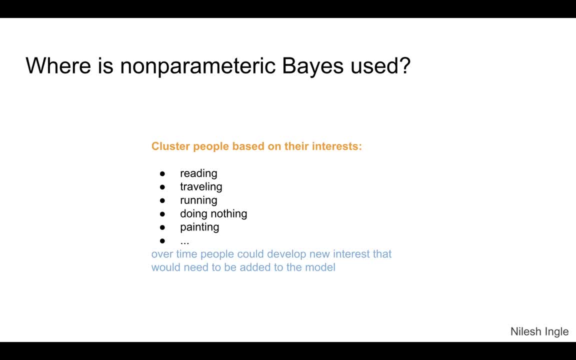 of a particular group of people, of a particular group of people in a cluster, represented by a cluster in a data set, is reading, traveling, running, doing nothing, just lying around or painting. there may be others as well now as the year progresses, if there are holidays, weekends, or if there are festivals, or if they have some other plans that come up. then their interests could change as the year progresses. so that's something we'll be looking at as we go along. 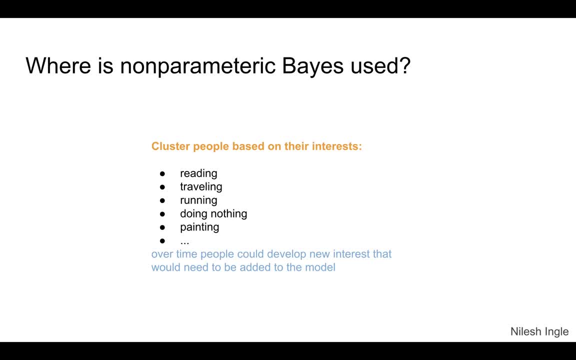 over time and so to in order to accommodate those new interests. we need a provision in the model that could handle that. otherwise we would have to go back and retune everything from scratch and then to account for each of those new clusters that come in to the data set. so non parametric base helps us. 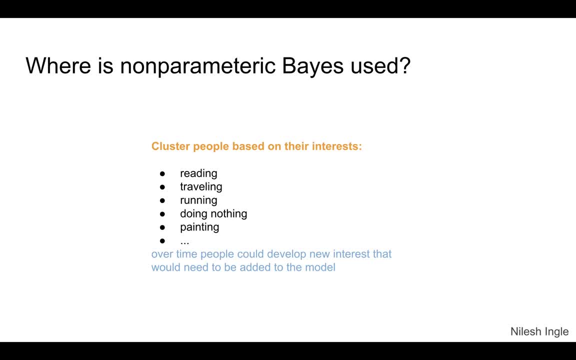 in those situation which can handle infinite number of clusters. so we do not have to specify the number of clusters ahead of time, although in scikit-learn we do need to specify the maximum number of clusters, just so that the algorithm would then stop at that point. and here are a couple of definitions: 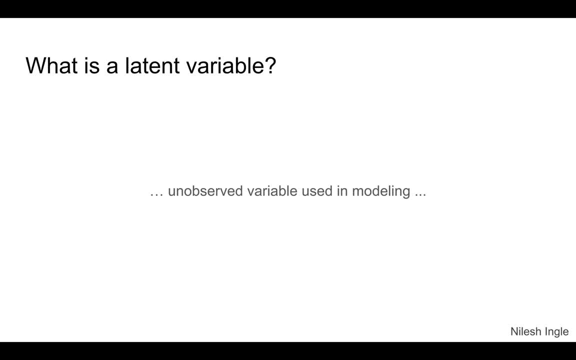 what is the latent variable? a latent variable is a variable that is unobserved. so earlier we saw that Z was the latent variable which was representing the clusters. so if we do not know what clusters are there, so that's kind of latent variable. now let's look at the difference between binomial and multinomial. 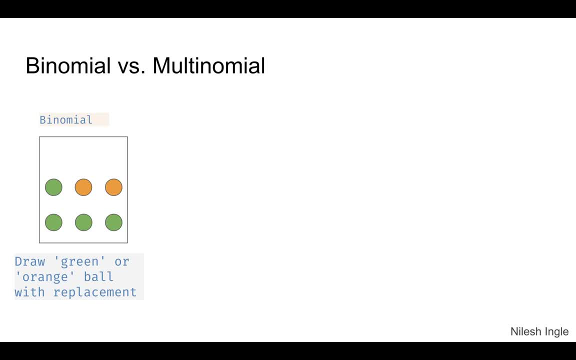 the reason why we are looking at this is because the Dirichlet distribution is based on the multinomial distribution. so in binomial we can imagine a box which has two types of two types of balls. we have green colored and orange colored, so we can draw a green or orange ball from this box with replacement for normal. 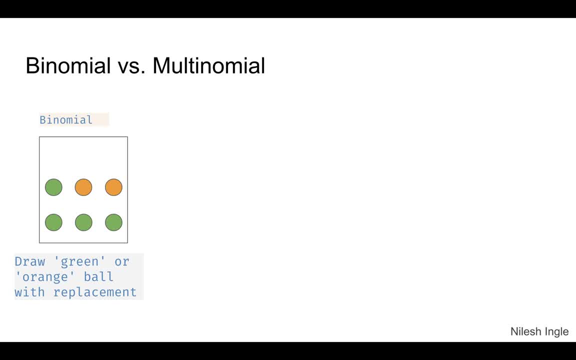 so we can draw green or orange ball from this box with replacement for normal. that would be like a binomial case, Multinomial case: we can have any number of colors in the box and we could have any number of balls in the box. 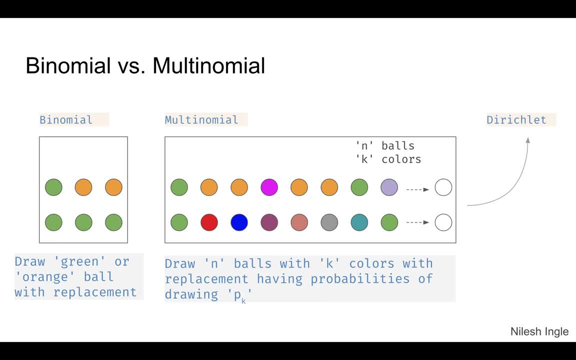 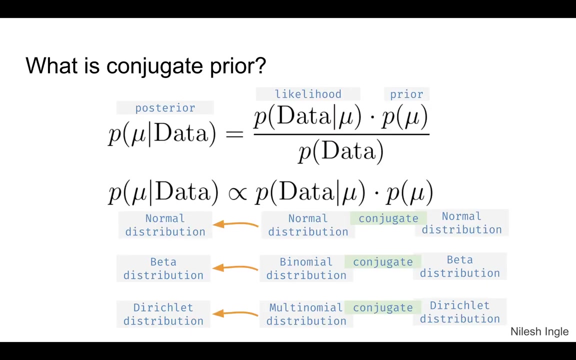 So we can draw n balls with n colors from that particular box and we'll have a probability value associated with that and Dirichlet distribution is based on that idea, So it's an extension of the multinomial. Another term that I will be using in this section is: 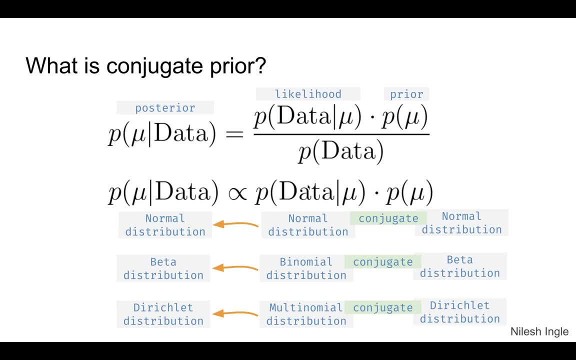 conjugate pair. What do I mean by that? Now, here we have this Bayesian formula, We have the parameter that we are trying to find based on, given the data is equal to this likelihood into prior upon evidence, And if you look at the proportions, if we skip this denominator, then we have this: 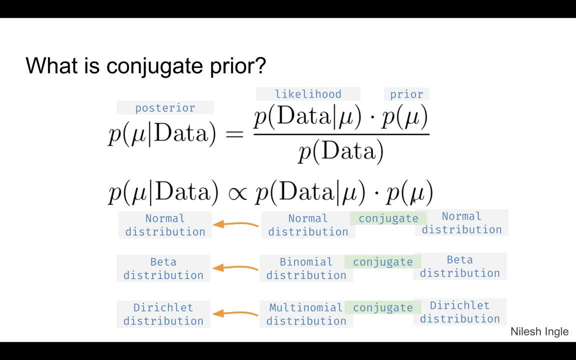 posterior is proportional to likelihood into prior And the conjugate pair is between, let's say, in this case, the normal, the prior is a conjugate And the conjugate pair of likelihood. if these are normal distributions and what that does is the output that we get, which is the posterior, is also the same distribution as the prior. 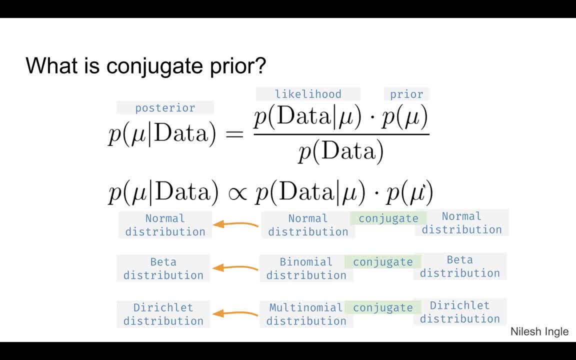 So, when we update our prior belief after seeing the data, the distribution that we have, the updated distribution that we have is also of the same type, so that's easier to work with as it's in the same type of distribution. so again, this is a beta distribution, is a conjugate prior for binomial, and then we have 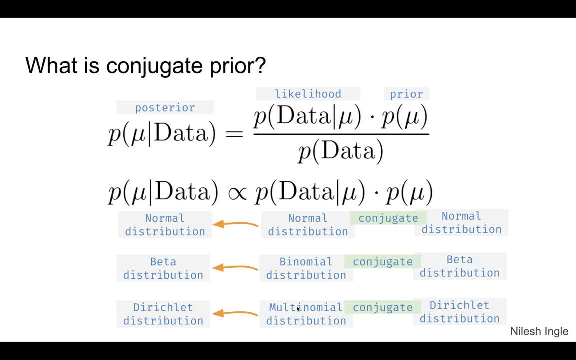 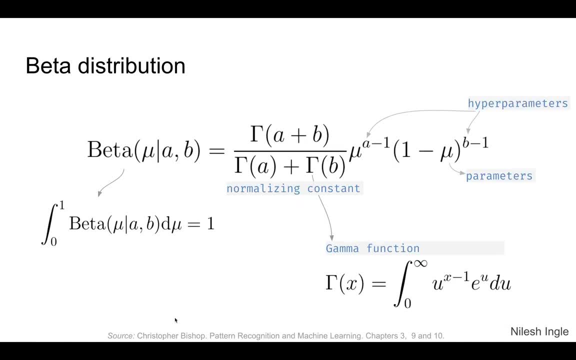 distribution that is a conjugate prior for the multinomial distribution, so the posterior is also Dirichlet distribution. so far now the beta distribution and will be. this is a very important distribution here. this shown by this particular relation right here. for moment we can ignore this term, which is a normalizing term, that is, to bring the 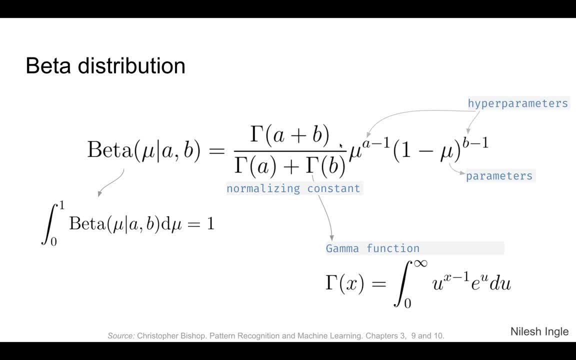 values between 0 and 1. we look at these. on the right hand side we have the parameter mu. so this mu is not the mean, it's the parameter. and then these two are the hyperparameters and the gamma from this capital gamma gamma is given by this relation shown here. 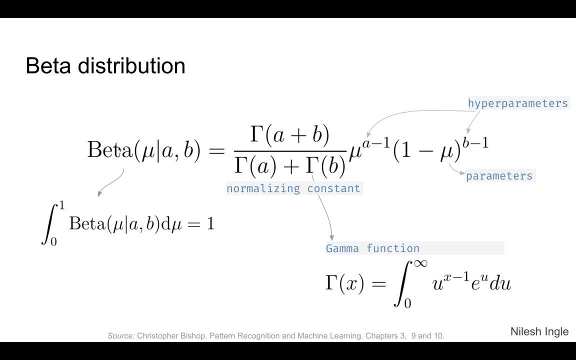 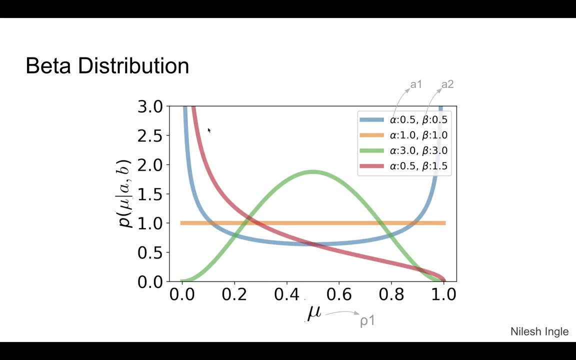 down below and for the values of this distribution. when we integrate it from 0 to 1, it should integrate to the value 1 and this is how the distribution looks like. we have the parameter mu on the x-axis and the probability on the y-axis. 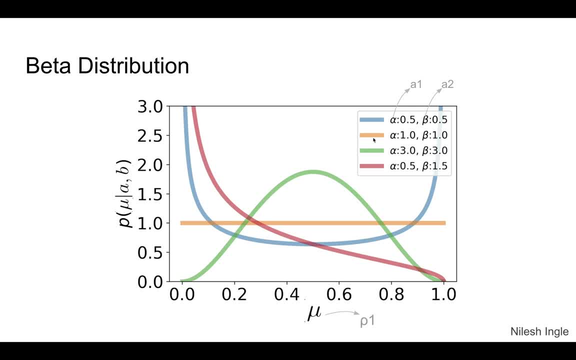 probability values on the y-axis and we can see that when the value of the parameters alpha and beta, which is a and b here, that those are one, then we get a horizontal line so that showing us a uniform distribution. then we have set them to a lower value of 0.5, 0.5. then we get this blue curve which is like a. 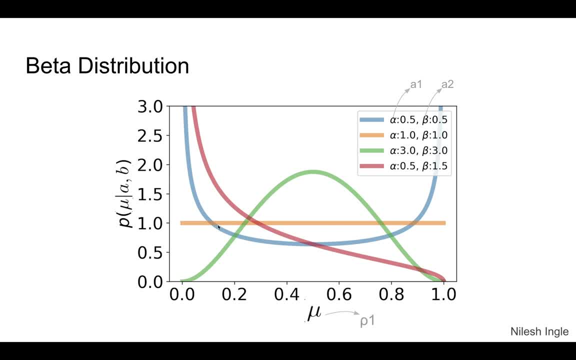 u-shaped curve, which is kind of pushing the values towards the edges as 0 and 1, and then we have the other shapes that are based on other values. you'll see that I'll be switching the notations based on the sources that I've referred to, but I'll try my best to mention them by showing them with the. 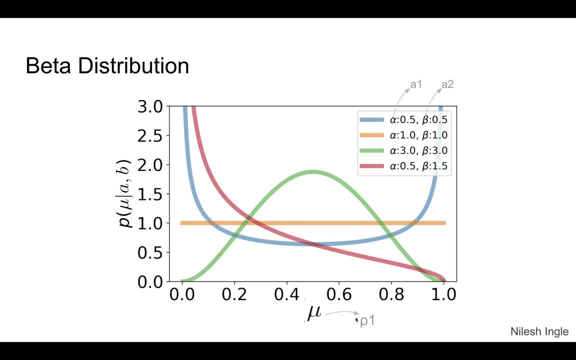 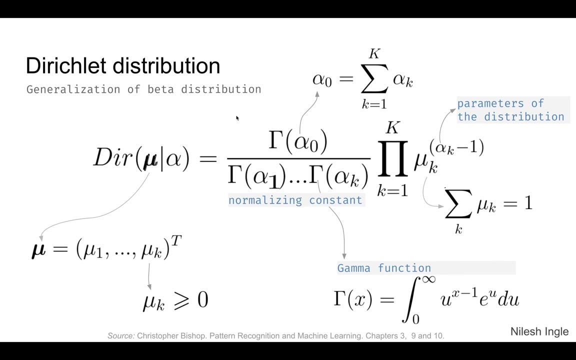 arrows right here. so this mu is also mentioned as rho in future slides and this alpha beta, in this case previous slide, we saw that this was a and b. in future slides we would also be referring to them as a 1 and a 2. and then we have the notation for Dirichlet distribution, which is a. 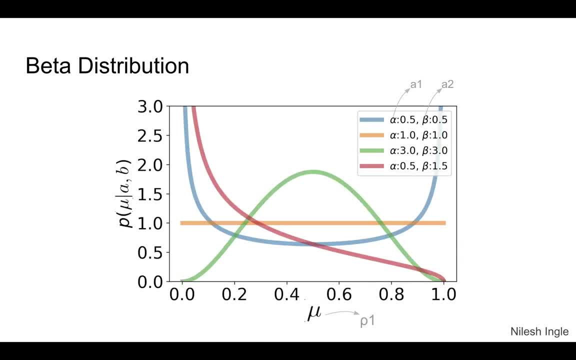 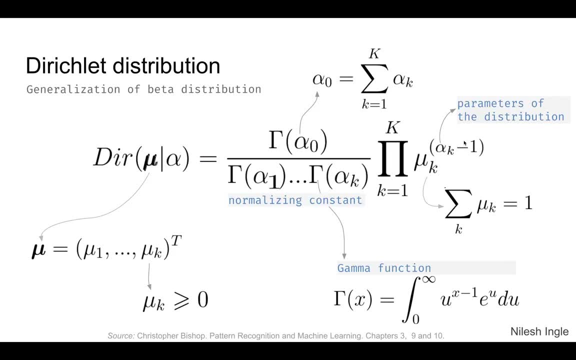 generalization of Beta distribution. so the beta distribution, like we see here, we have two parameters, a and b, two hyper parameters. in Delta欸 distribution we can have any number of hyperparameters. so which is shown here by alpha k, and again this is the normalizing term right here, and we have 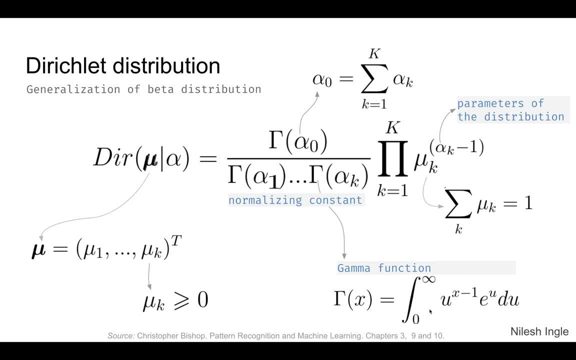 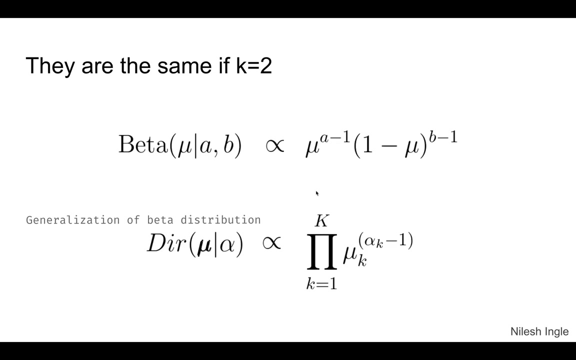 the gamma represented by this notation shown here, and that's a mathematical form for the Dirichlet distribution and we'll be using this in what is called as a Dirichlet process. and this is a comparison without the normalizing term and, as you can see, two. 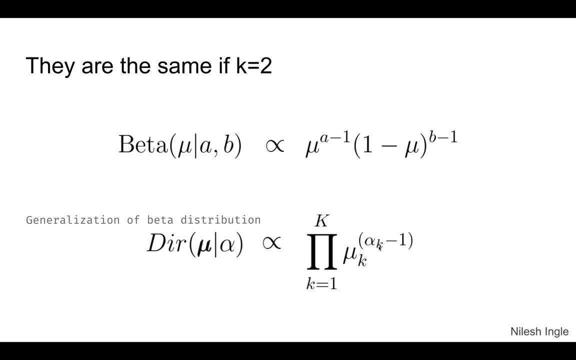 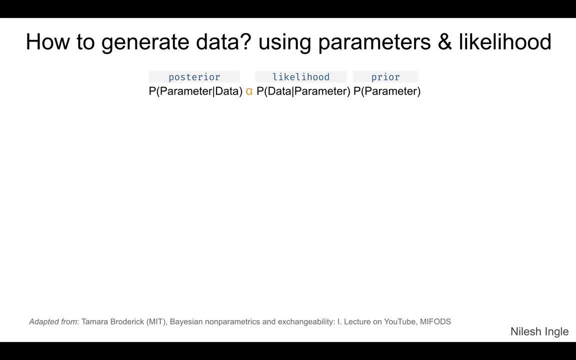 hyperparameters, and here we can have k hyperparameters. now let's look at how we can, let's look at the Dirichlet process, how we can use the beta distribution Dirichlet process to generate data, and how we can use the beta distribution Dirichlet process to generate data. 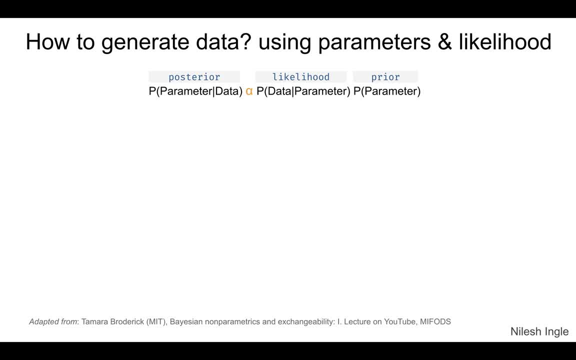 to assign data points to a particular cluster. so again, we start out with this in our background, which is the posterior is proportional to likelihood multiplied by prior. what that is telling us? that we start out with prior values for a parameter that can be drawn from a distribution such as a normal distribution. 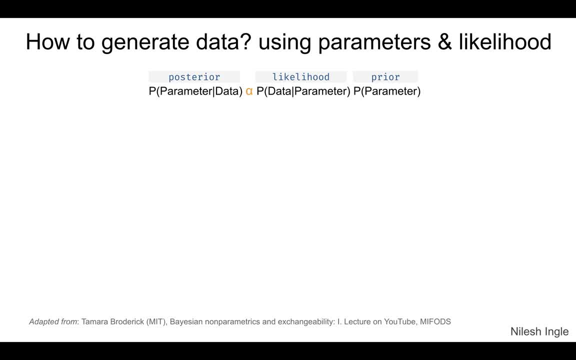 and then what we want to see is, after looking at the data, how those parameters get updated, and that's that would be our posterior. so here, let's say we have two clusters, shown by the orange X and the green X, and the primary cluster is a lot of data, which is an 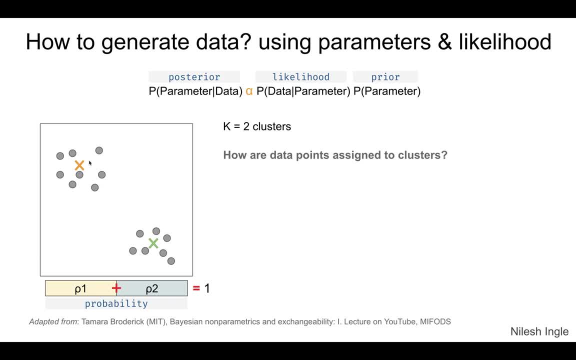 of data points. each of these data points associated with this distribution right here and this distribution down here is represented by row 1 and row 2, and so those add up to 1. total is 1. so how are then the data points assigned to these? 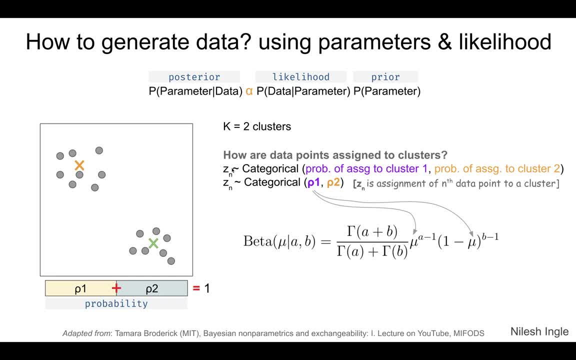 each of these clusters. so we have, we create a variable Z of n. what that variable does, is it? it is, let's say, it holds the values of probability of each of the data points for the values of probability. that though that data points for the values of probability, that though that. 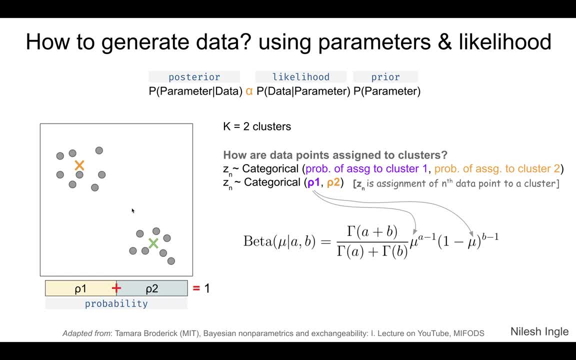 comes from the distributions that represents the clusters. so what that helps in doing is it helps assign a particular data point, either to cluster a or cluster B, either to cluster this cluster or that cluster, or or. in other words, we have the values of probability, probability so we can say to what extent a particular data point would. 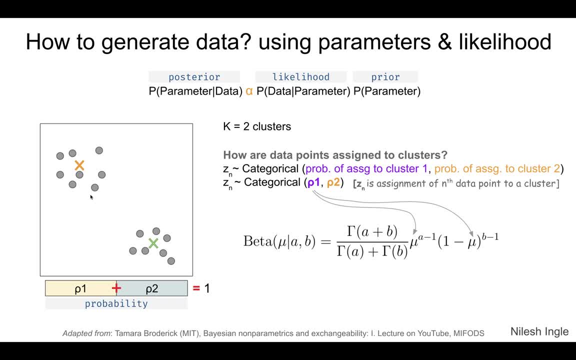 belong to a cluster which is represented by orange or which is represented by the green X right shown here, and those values for the row which is comes. so here we have the the row which is comes. so here we have the the row which is comes. so here we have the. 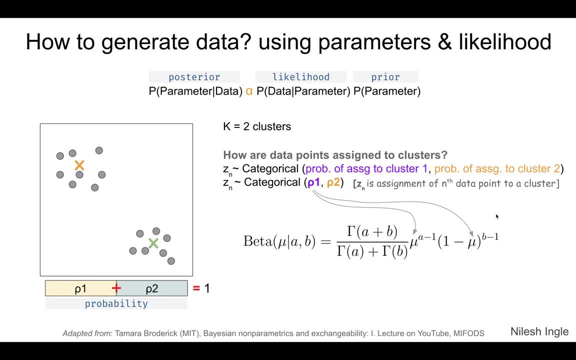 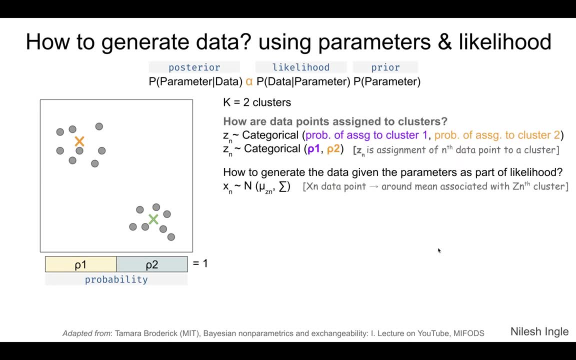 mu representing shown here in this equation. so that is the same as rho. so both of these mu would be rho 1 and we can then use the beta distribution to get those values. next we can look at how we can generate data given the parameters. part of likelihood, so here: 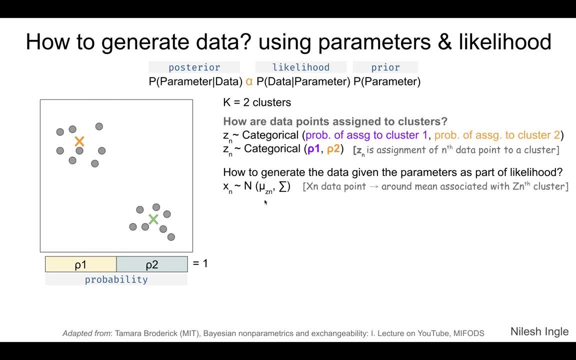 we can get the values for xn from a normal distribution with a mu, with a mean mu for that particular zn cluster, for a specific cluster, and the covariance for that particular cluster. now, in this particular case, what we do not know is the mean or the mean of each of these clusters. 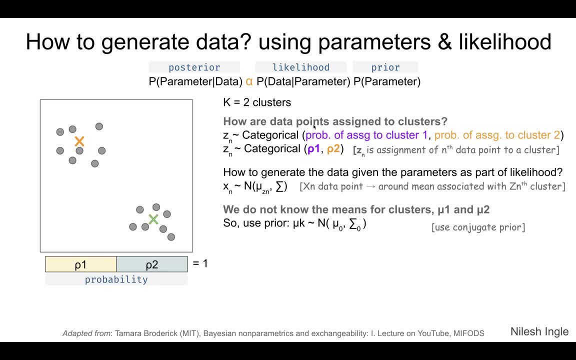 so to start with. so those are the parameters. so to start with, what we can do is sample them as a prior from a normal distribution. so, as shown here, we can use n normal distribution with mean of mu 0 and sigma and covariance as sigma 0. 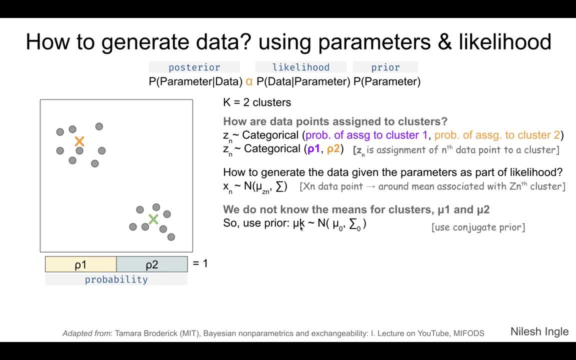 to sample the prior mean and covariance for each of the clusters that would be represented by mu k. so here we would have the 2 mu 1 and mu 2. secondly, what we do not know are the probability values rho 1 and rho 2, and we can get those. 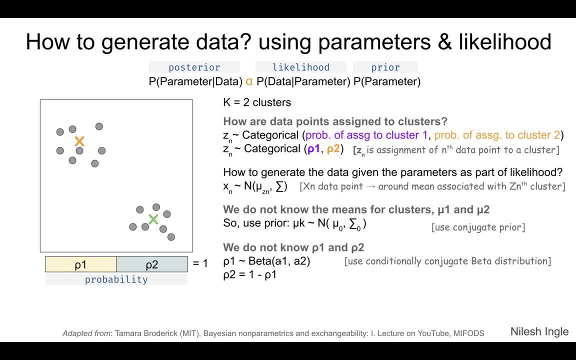 values from the beta distribution. so to the beta distribution distribution. we would import a1 and a2 parameters to get the values for the probability rho 1 and then rho 2. we can calculate it by subtracting rho 1 from 1 and the uh, the total of these would be 1, and the reason why we just have 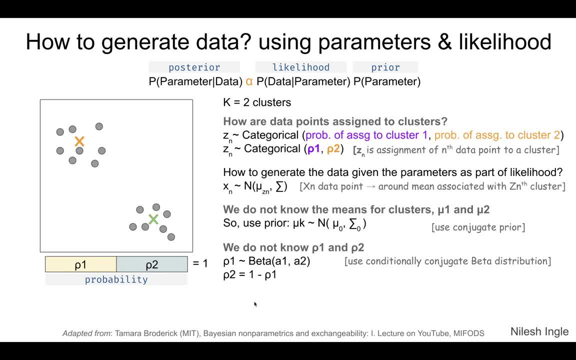 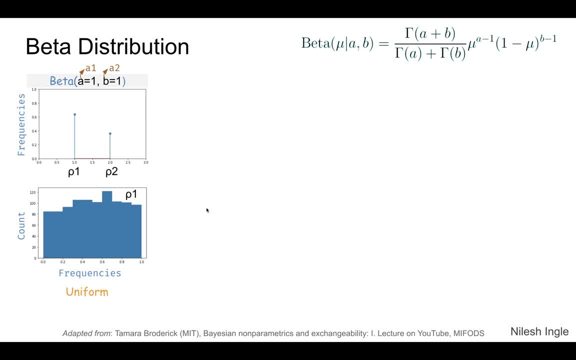 rho 1 and row 1, row 2 and not row 3 is because we just have two clusters. Now here are some interesting plots. So the relation that is shown here up top the hyperparameters are shown as a and b, and that's what I've. 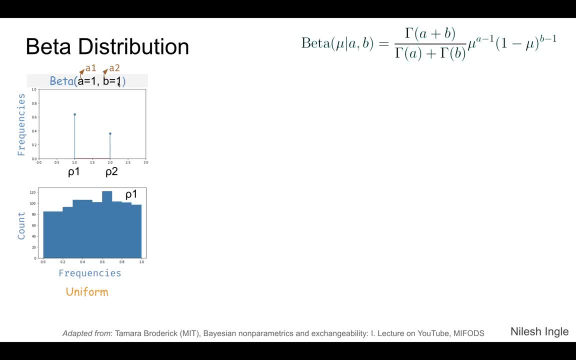 written here: a is equal to 1, b is equal to 1.. However, in the previous slide I've shown them as a1 and a2.. I hope that's not too confusing. So the very first plot on top here what we have are the values for row 1 and row. 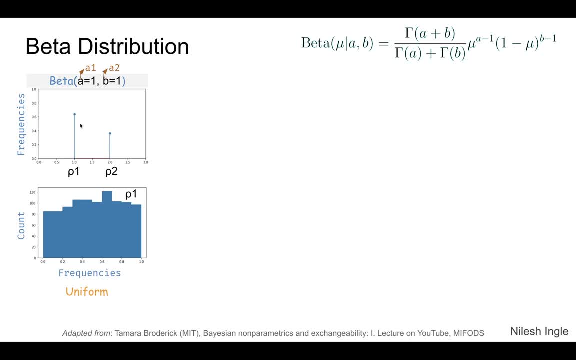 2, which add up to 1.. At least they should. We have this value that's slightly above 6, 0.6, and this value is a slightly below 0.4.. So that should be close enough, And what these are telling us is: this is just one sample for from the beta. 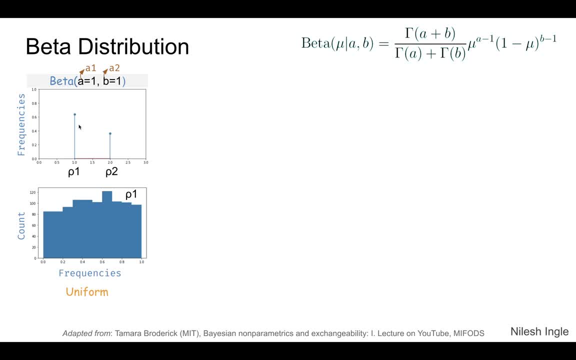 distribution. that is telling what the priorities would be for a data point to lie either in cluster 1 or cluster 2.. If we sample row 1 several times, maybe hundred or thousand times, and we try to plot the distribution, the distribution looks like what we see here in the bottom. 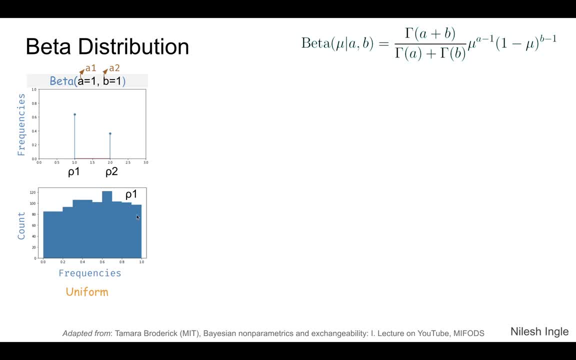 histogram and it's close to a uniform distribution. Not exactly, but close to a uniform distribution. Now, if we change the values of the hyperparameters a, b to 0.01, 0.01, that is to say we have reduced, and then we are reducing the inhibitez. 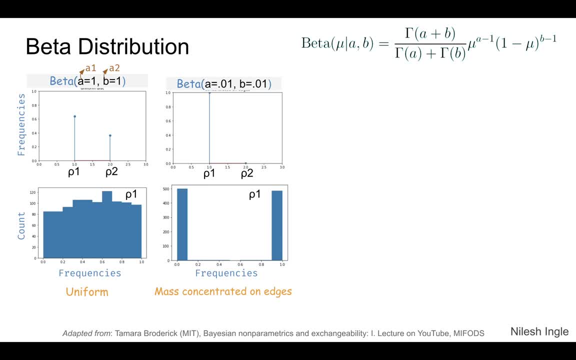 using the radical imaginary distribution that boarts the input and that We are inputting very small values. In that case the priority shifts to he shift to the cluster, row 1.. In this case, and if we try to plot the histogram, if we sample the histograms several times, 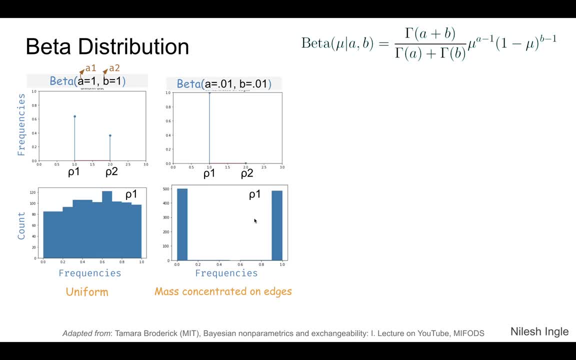 and if we try to plotope the histograms 7.15/ is because the probability is shifting to the edges and that's what we saw by the U curve in the distribution plot and that we saw for beta distribution in earlier slides. that's shown here. so we have peaks at 0 and 1 and then this as: 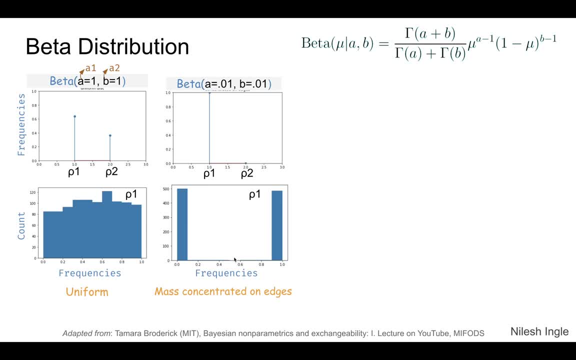 there are bars right here, but they are on the height of them, those bars is very, very small. Then, after this, if we, on the flip side, if we increase the value of the hyper parameters for the, which are the input to the beta distribution, you see that the values of probability for row 1 and 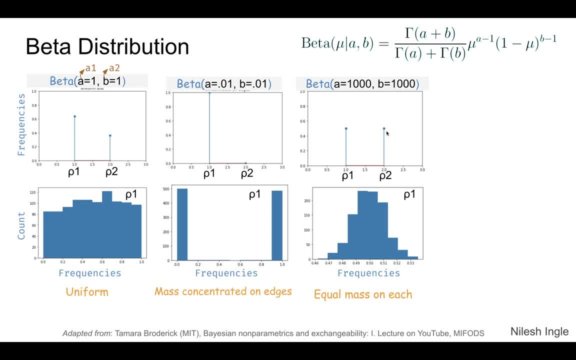 row 2 are similar, so it's like equal weightage is given to both the clusters and we sample row one, let's say, several thousand times or several hundred times, and if you plot them we get a distribution which looks like a normal distribution, as shown down here. so it's telling. 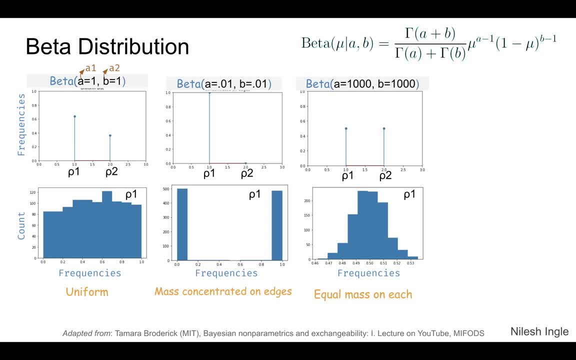 us that there is equal mass on each of these. so these could be the points that are on the decision boundary of the between the two clusters. and finally, we have a situation where the value for the hyperparameter a is higher, much higher than 10 times higher than the value for the. 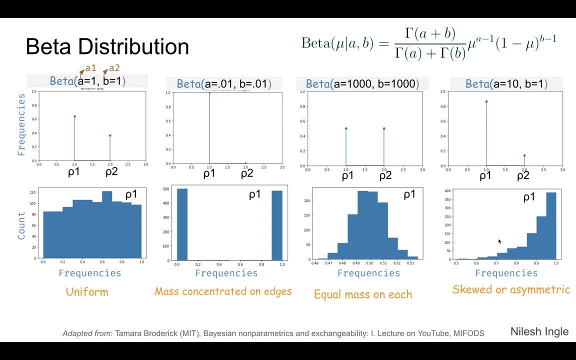 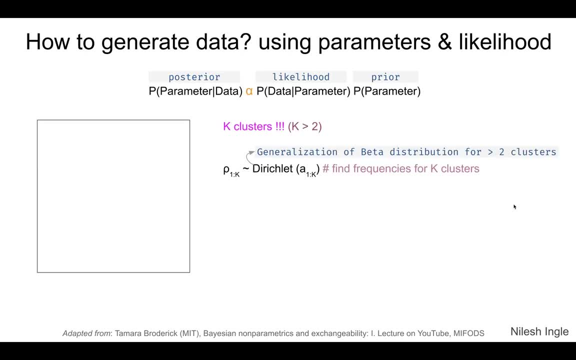 parameter b and we can see that the final histogram is skewed and it's not symmetrical. now, so far we looked at what we would do if there were two clusters. what happens if the number of clusters is more than two? that's where the Dirichlet distribution comes in. 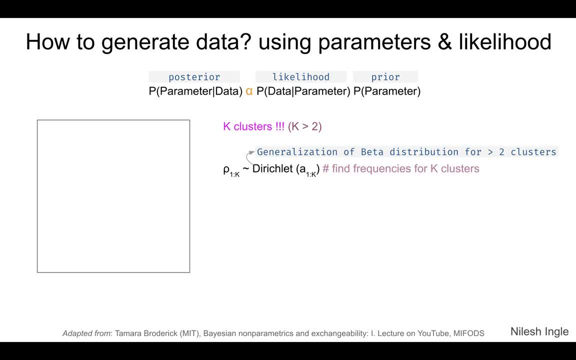 and Dirichlet is a generalization of beta distribution, as we saw earlier. so we have more than two hyperparameters because we have more than two classes now and it is given here. so the probability that we would get from a Dirichlet would be from 1 to k. so on those minimum number of probabilities we can get, 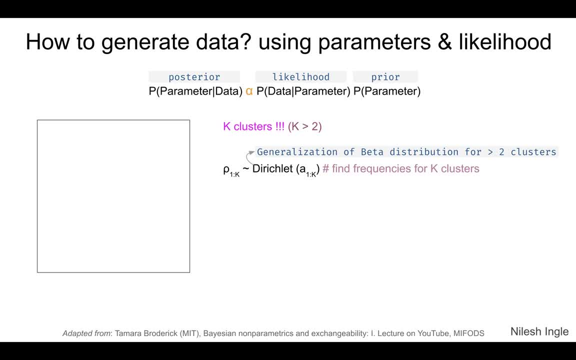 as many classes there are in the data set. so here we have input of hyperparameters. so the number of hyperparameters again would be 1 through a k, or 2 a k, based on how many clusters are there to be found. and so that's what we discussed. now, row k again, should the values for 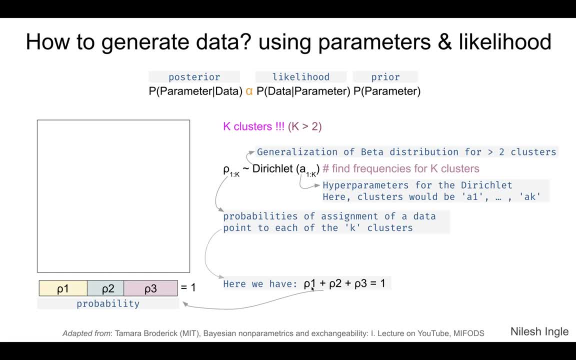 row should again sum up to 1. so if we have three clusters, the value of row 1, row 2, row 3 should sum up to 1. and now for the values, for the means. we can sample them again from a prior conjugate. here it is shown by a normal distribution with mean mu 0 and covariance. 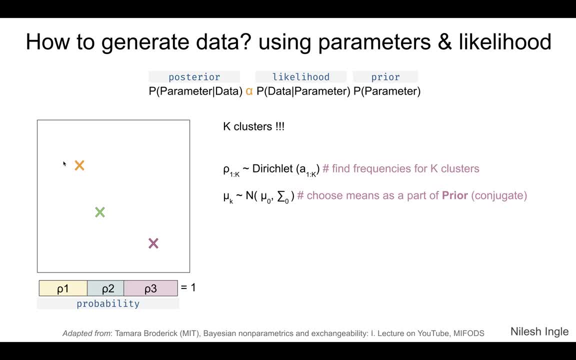 sigma 0, and those means are represented here by the x's for each of the clusters. now again, as before, we have Zn which can be used, which can choose assignments for data points to clusters, and that is done based on the values for probability row for each of the clusters. 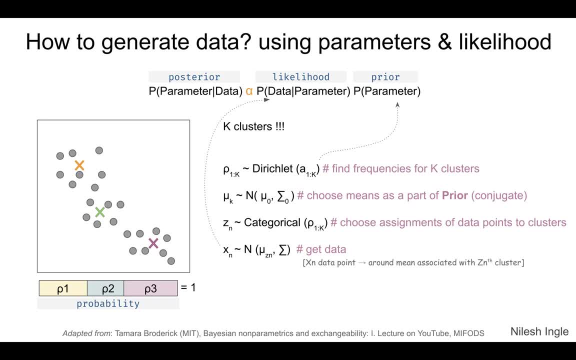 and finally, to get the data, we can use the mu, the mean for the cluster to which the data point would be assigned, Zn, and the squared and sigma, and those are tied into the relation that we have up above, which is the likelihood and the prior. so again here on the left hand side, we would have these data points allocated or associated with the distributions. 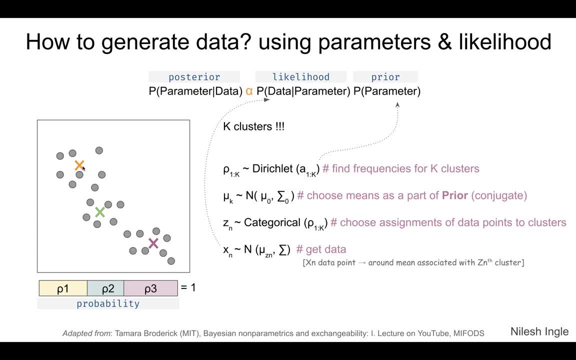 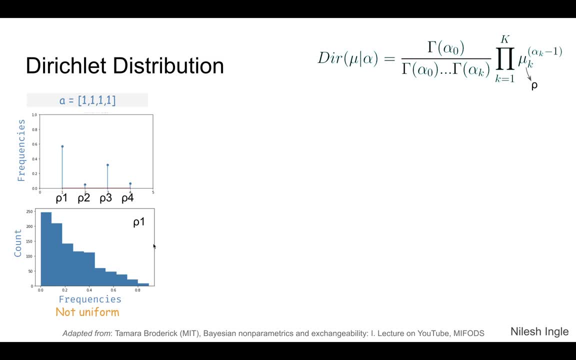 that are represented by the mean and variance associated with these Xs. Now to visualize the Dirichlet distribution we have on the left hand side in this particular plot, we have four classes, so sorry, four clusters. and when we set the value of hyperparameter A or alpha to 1, all of them 1, then we get a distribution, a discrete distribution, such 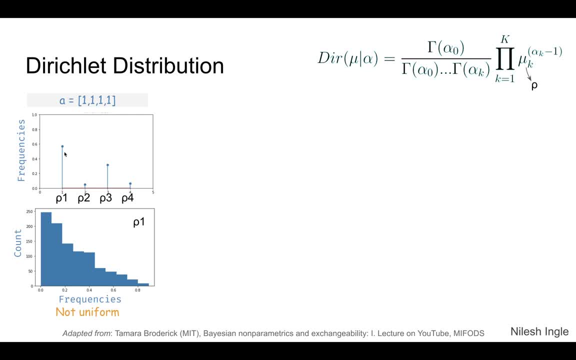 as shown here, and if we pull just row 1 and sample it several times, we get a distribution shown down below, which is not uniform as compared to what we saw earlier for the beta distribution, which was very close to The uniform shape, again as similar to the beta distribution in case of a Dirichlet distribution. 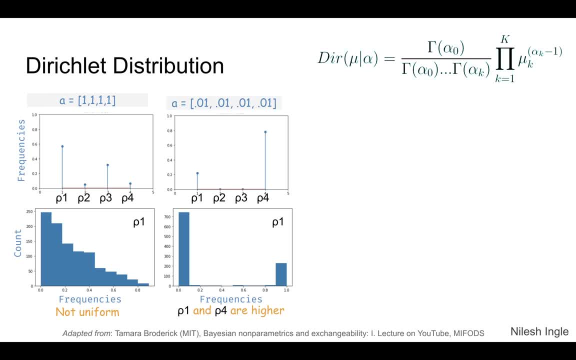 if we reduce the value of the hyperparameters to, let's say, 0.01, then we see the similar behavior as we saw with the beta distribution, where the quality mass gets shifted to the edges. And so Here we have row 1 and row 4 that have probabilities much higher than 0. the rest 2 are closer to. 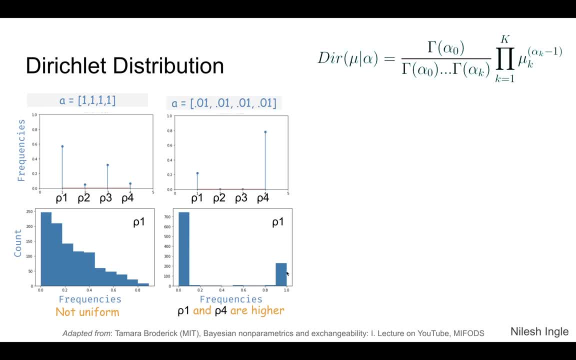 0 and if we sample row 1 several times and plot it, we see that 2 bars at 0 and 1.. And again, similar to the beta distribution. now, when we sample from a Dirichlet distribution with the values, The values for hyperparameters, which are much higher. so if we set it to 1000, then the 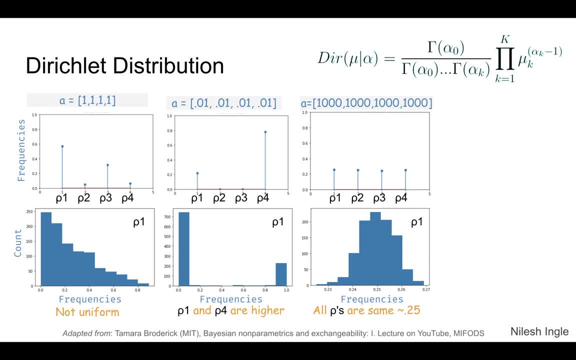 probability values for the row 1, row 2, row 3, row 4 are similar, so in this case there would be 0.25, and if we pull row 1, sample it several times, we get this nice Gaussian looking curve Distribution For the probability distribution.